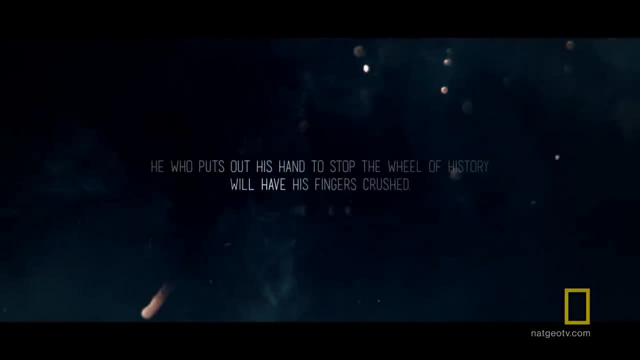 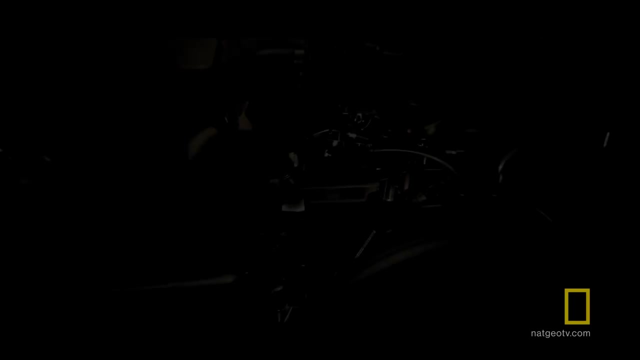 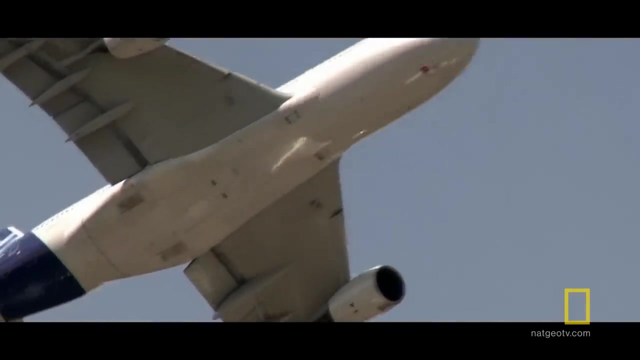 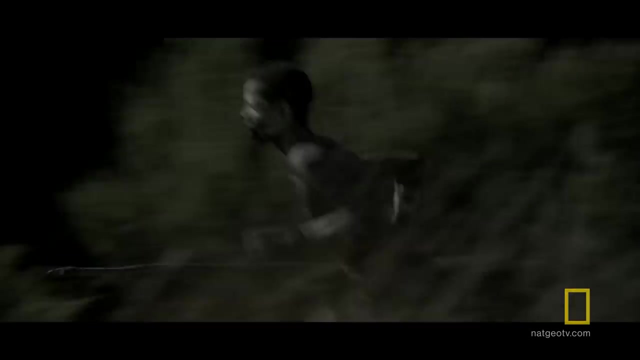 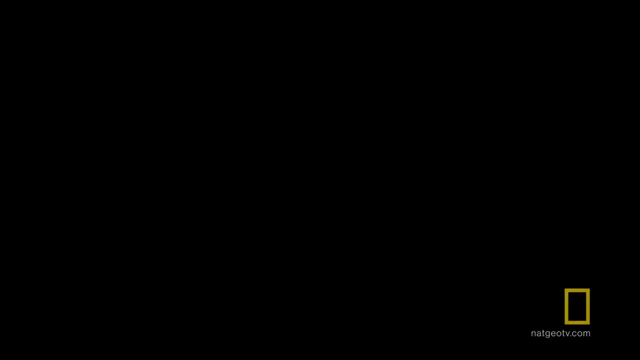 What does it take to power a global civilization to connect billions of people across continents? It takes the power of transportation. From the beginning, speed and strength were paramount In the hunt on the battlefield. we're holding together far-flung empires. 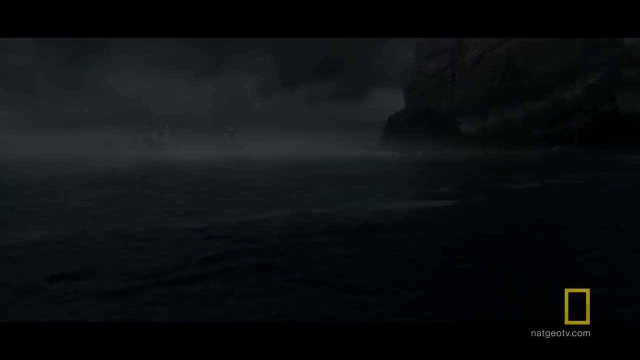 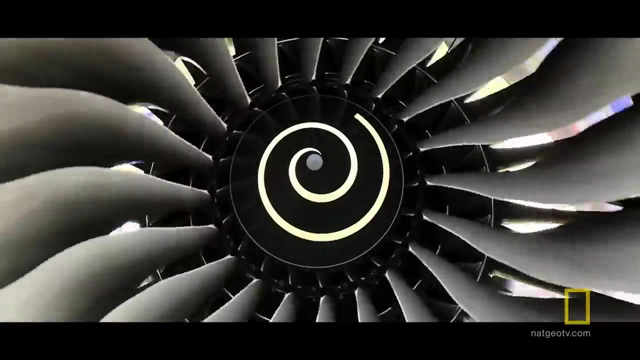 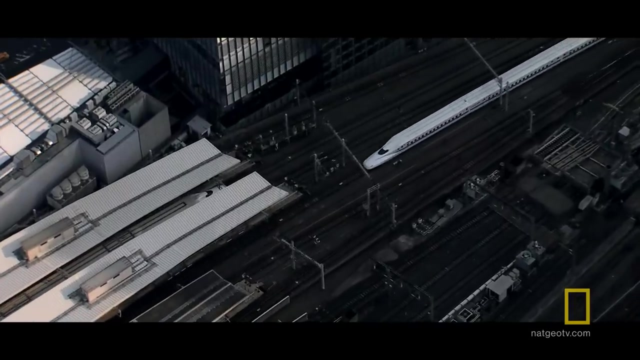 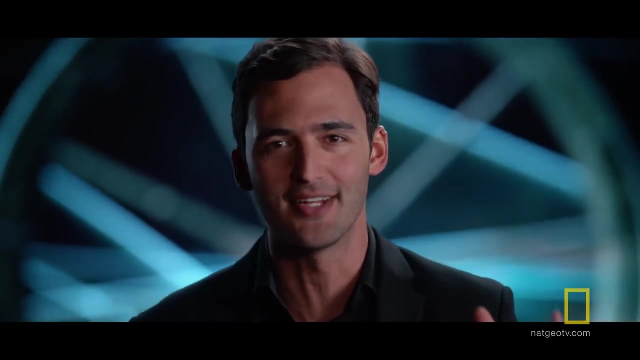 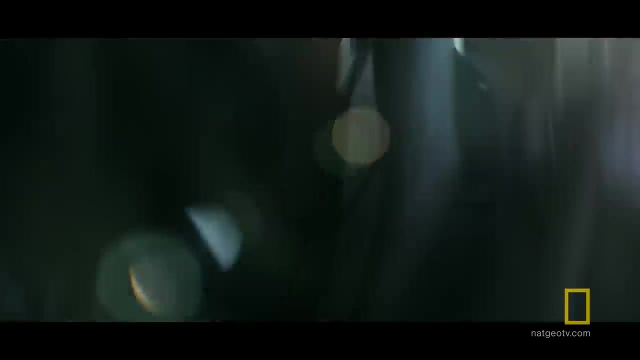 We sought new forms of power, harnessing the forces of nature to drive us forward: The horse, the wheel, steam power, jet engine. Every new innovation powered our next great leap. Transportation has become our exoskeleton, allowing us to transcend our biology. 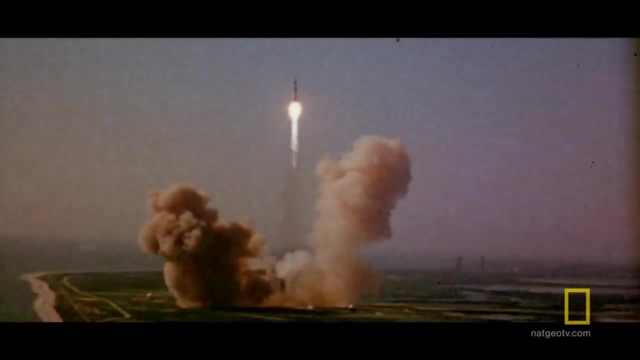 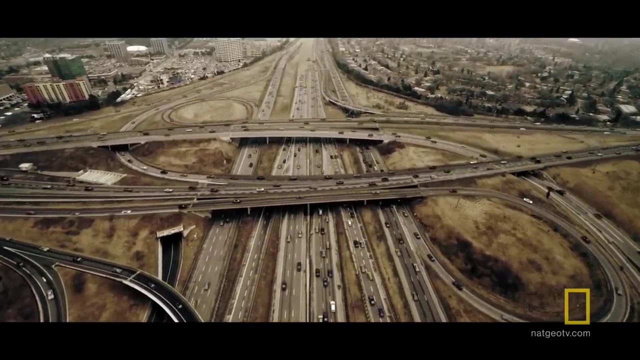 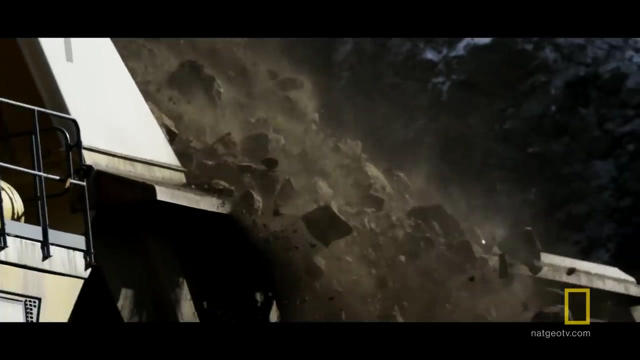 Faster than sound, Farther than the moon. Our inventions give us a level of power we never imagined. With our machines, we carve through solid rock, Tunneled beneath the seafloor, connecting the world, mixing distant cultures. Freedom of movement has given us freedom of mind. 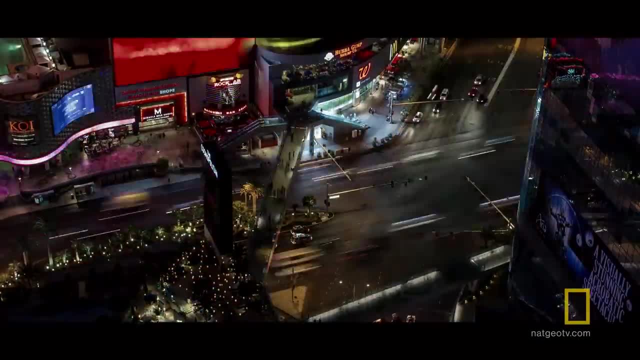 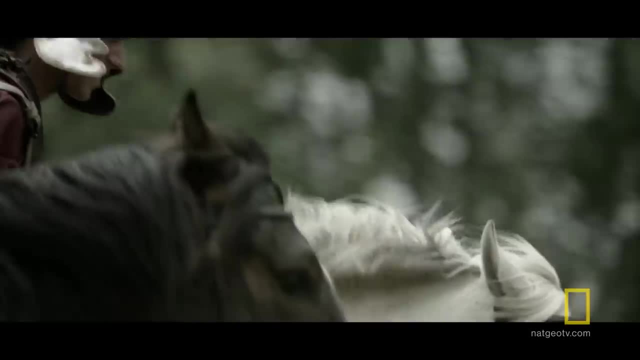 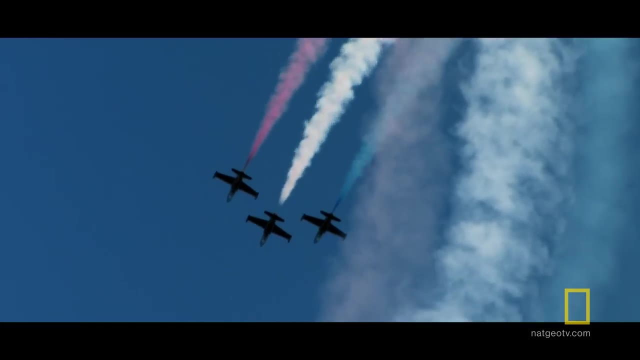 The flow of people and materials exposes us to new ideas and new understandings. This is the story of how transportation turned society inside out, How engines and animals powered the rise of civilization, How the innovations that drive humanity forward made us modern. This is Origins. 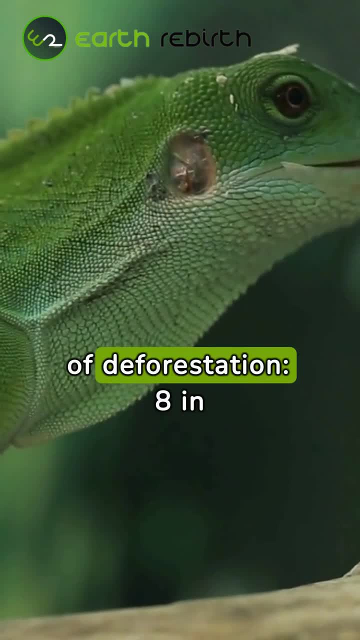 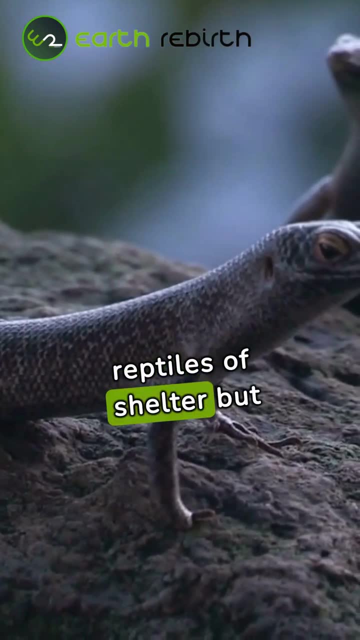 A recent study exposes a startling consequence of deforestation: Eight in ten lizard species are at risk. The loss of their arboreal homes not only robs these reptiles of shelter, but critically impairs their ability to regulate body temperature. Lizards which rely on the 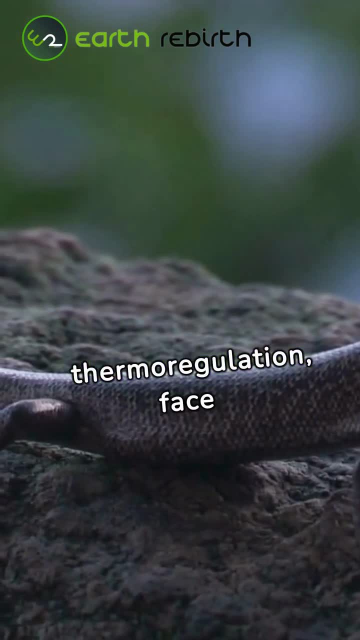 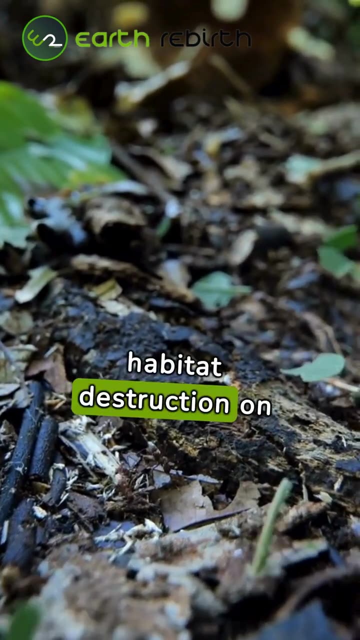 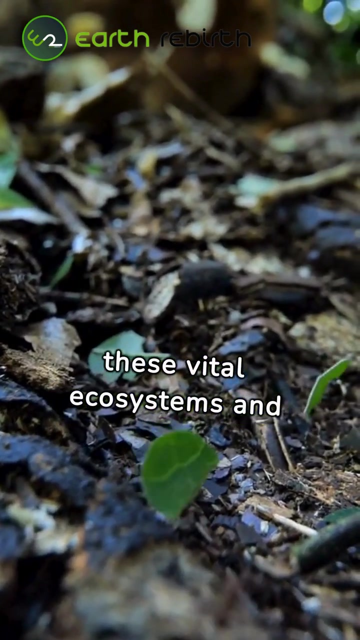 sun's warmth absorbed by trees for thermoregulation, face a dire future as their natural habitats dwindle. This study underscores the cascading effects of habitat destruction on biodiversity, sounding an alarm on the urgent need for conservation efforts to safeguard these vital ecosystems and the myriad life forms they support, Like, share and follow. Earth Rebirth.